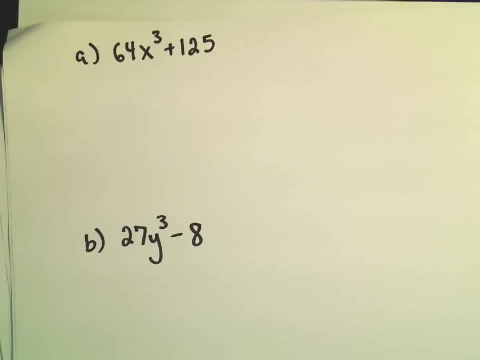 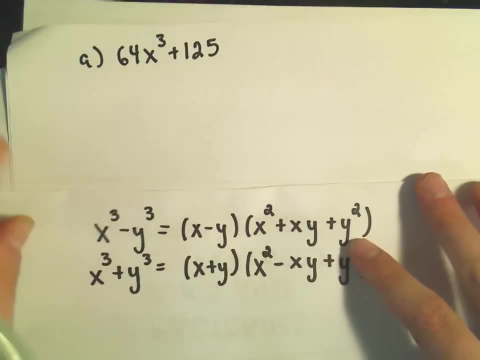 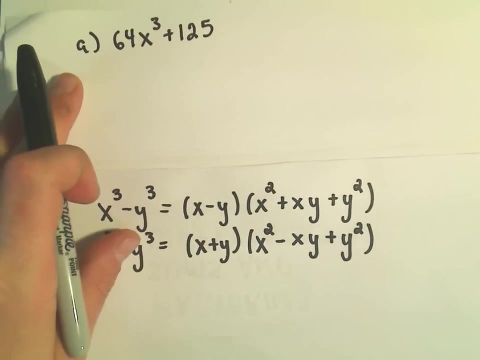 So let me see if I can bring my formula back in here real quick. Okay, so it looks like in this one we'll have to use the bottom formula. Okay, so it looks like we have something cubed plus something cubed, but the first thing I'm going to do is I'm going to just rewrite it a little bit. 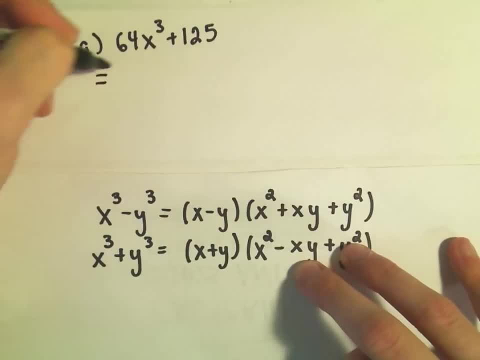 Okay, so I'm going to rewrite my 64x cubed And what I'm going to do is I want to write that as something cubed plus something else cubed. That's kind of how I'm interpreting this second formula: something cubed plus something cubed. 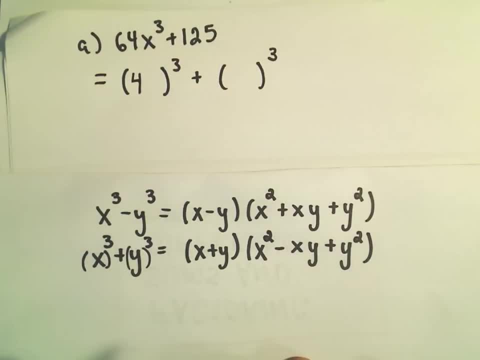 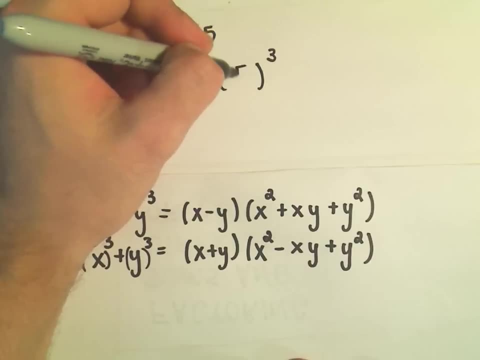 Well, I guess to get 64, we would need We would need 4 cubed, and to get x cubed we would just need to stick an x in there. Likewise, to get 125, we would need 5 cubed. 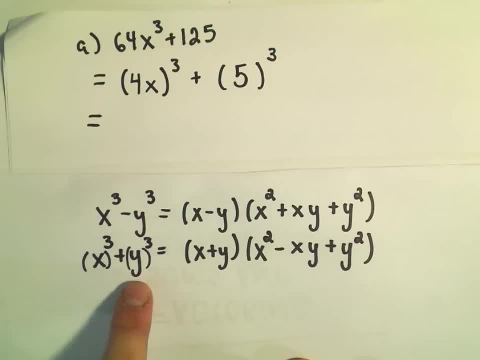 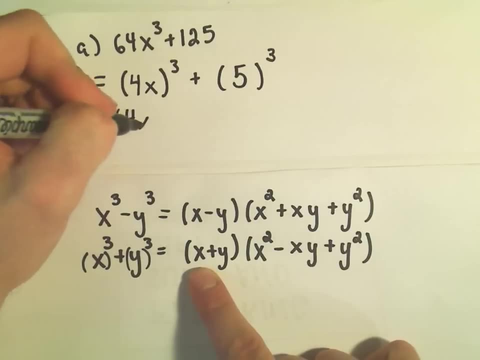 So now I'm going to use this formula. So instead of just x and y, I've got 4x and I've got a positive 5.. So instead of x, I've got 4x. and then it just says: write plus whatever's in the second set of parentheses. 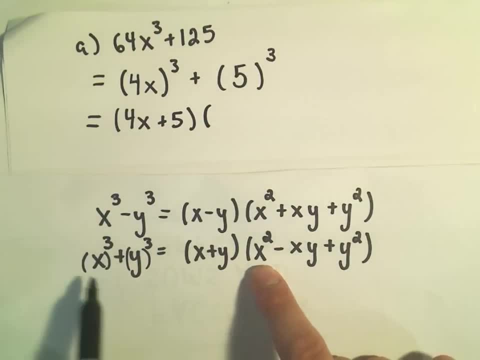 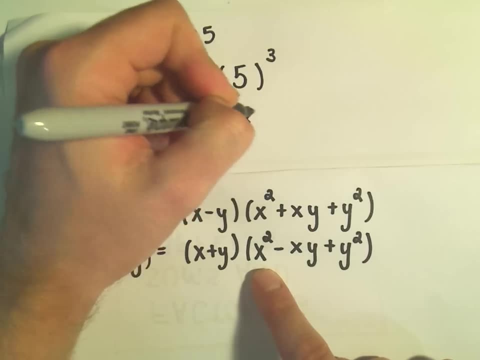 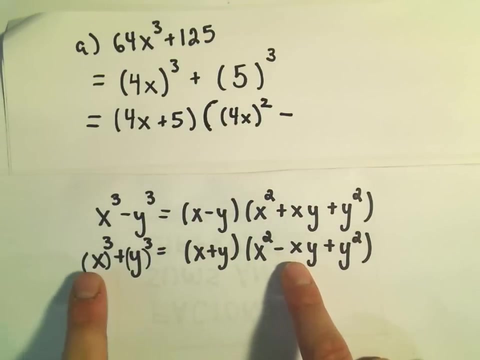 And then it says It says now take that thing and square it. So I'm taking my 4x and I'm squaring it. Then it says write a minus sign. It says take the first thing times the second one, So 4x times 5.. 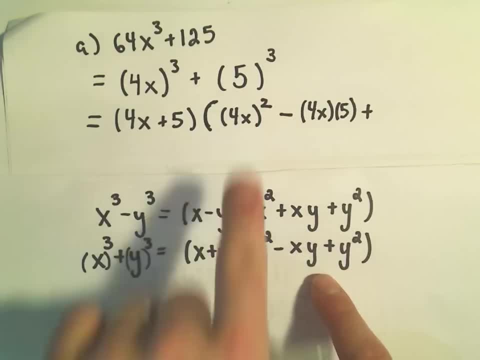 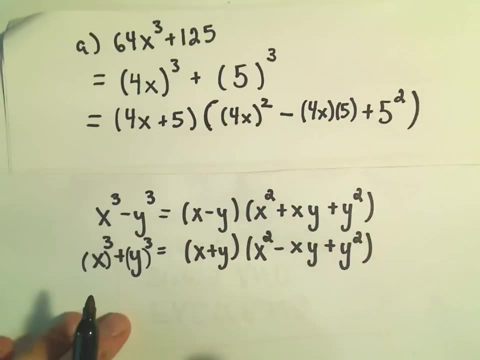 And then it says write a plus. and it says whatever number was being originally cubed, it says now we take that number and we square it. So certainly I think it takes a little getting used to. for sure, If we simplify this, we have 4x plus 5 in the front. 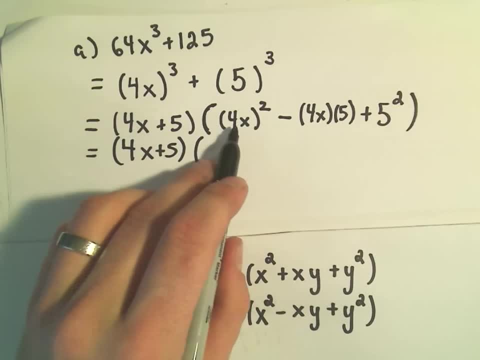 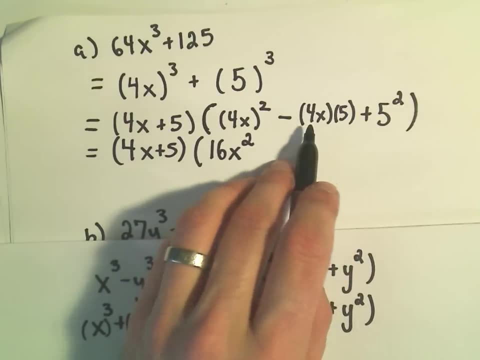 Not much to do there, And I'm going to take 4x and square it. So 4x times 4x would be 16x squared. We have negative 4x times 5.. Well, I can multiply the negative 4 and the 5 and make that negative 20x. 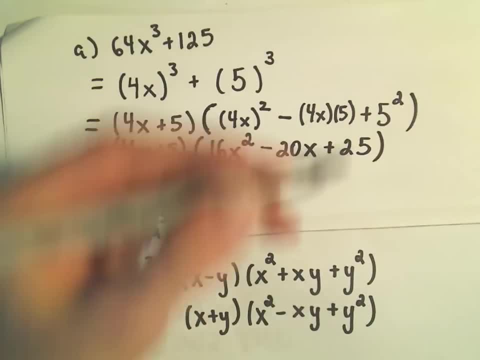 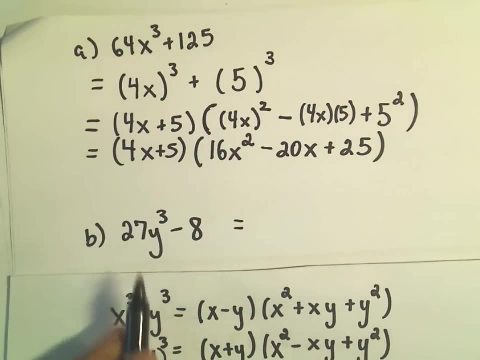 And then our positive 5 squared will just get positive 25.. Okay, So one more here I'm going to do the same thing. I have something cubed minus something, Well okay. So the trick is we have to again kind of rewrite them both. 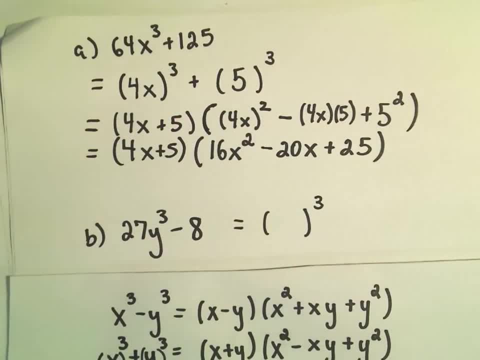 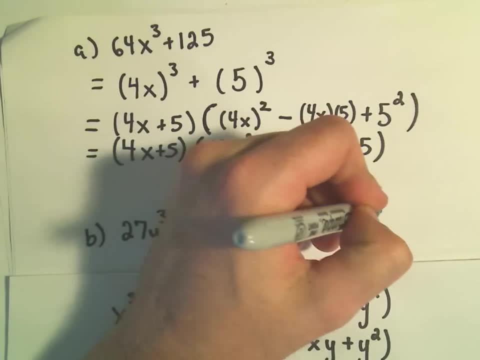 So I think what number cubed would give me 27?. And there we would just need a 3.. And to get the y cubed we would need a y in the parentheses, Minus. and now I think what number cubed is 8?. 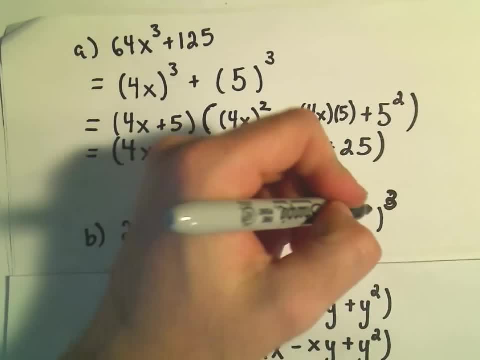 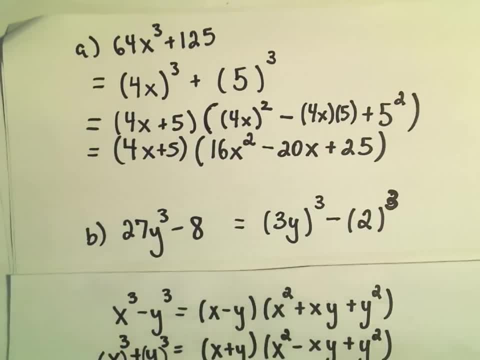 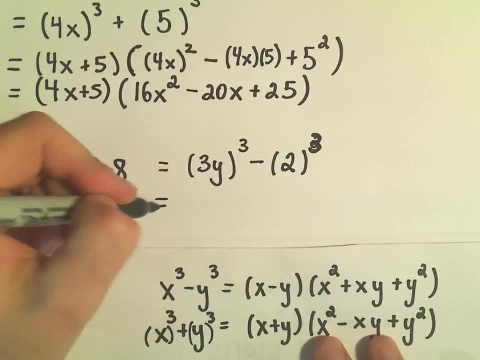 I think 2 cubed is going to give us positive 8.. And now we just do the same thing. We just use our little formula here. Okay, So don't get confused by the x and the y here and the fact that we have y's and numbers. 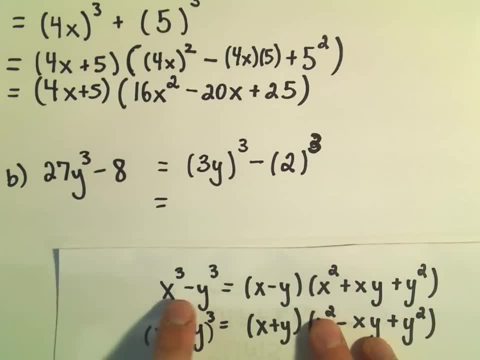 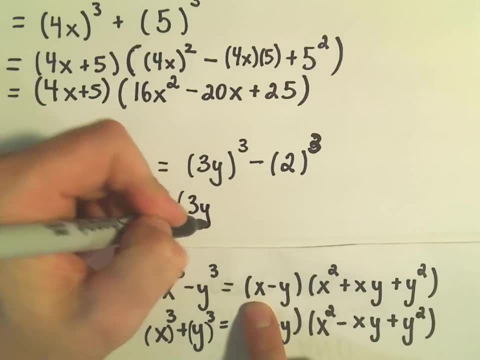 To me. we're using this formula And it says: if you have something cubed minus something cubed, it says whatever was being cubed, so kind of whatever's downstairs, write that first, So we'll get a 3y. 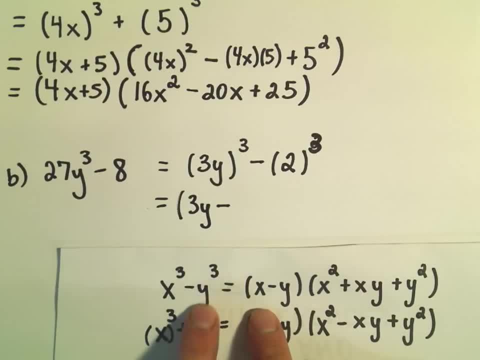 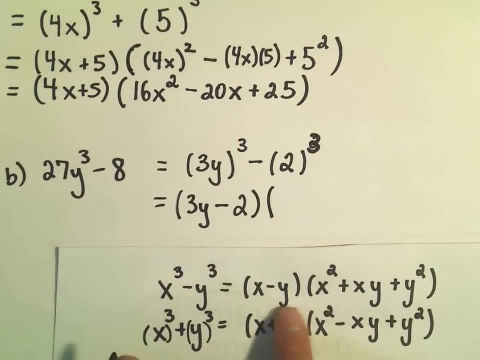 Then it says: write a minus sign. And it says whatever was Also being cubed. it says: just stick that next to it, So we'll just drop our positive 2 down. And then it says: take the first thing in the first set of parentheses and square it. 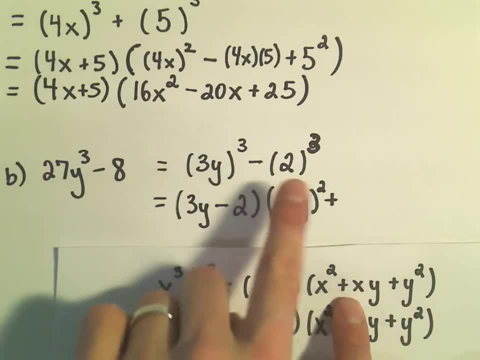 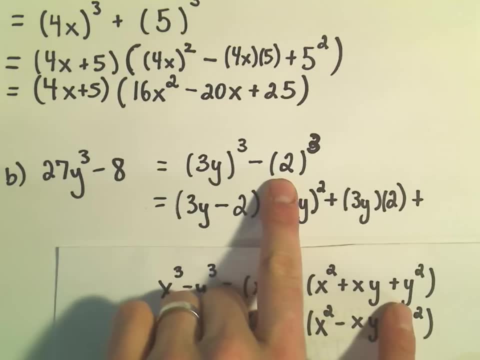 Then write a plus And now multiply the things inside the parentheses together, So 3y times 2.. And then it says whatever number was out there, it says we just square that as well, Okay, Okay. So if we simplify this, 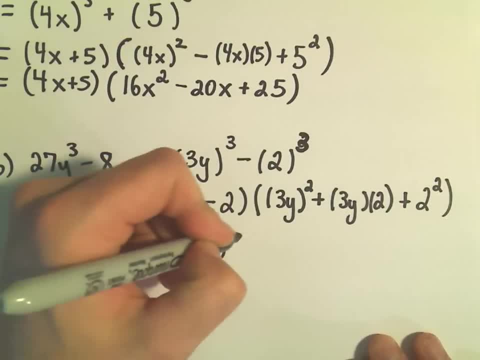 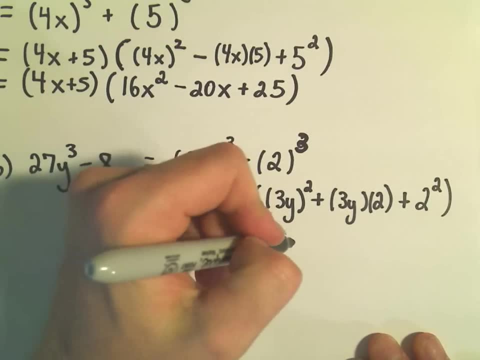 We'll get 3y minus 2.. 3y times 3y will give us 9y squared. 3y times 2 will give us positive 6y And then 2 squared will give us a positive 4.. 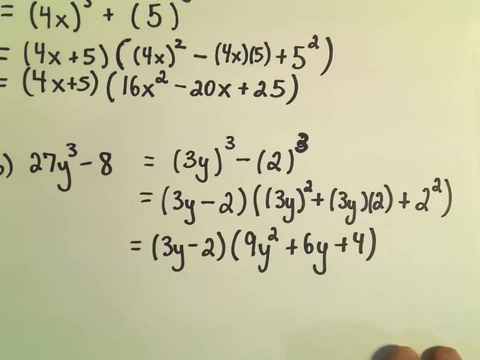 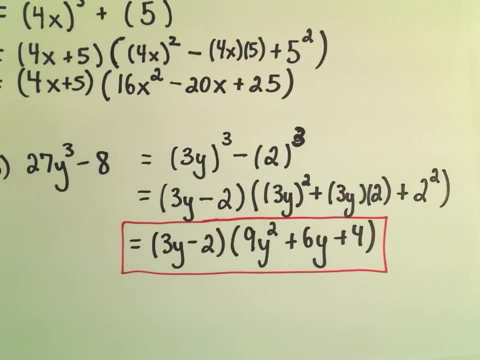 And again, we have now factored 27y cubed minus 8.. Okay, So again, I think these are formulas that you don't run into all the time. You'll see them a little bit now and again. you know in calculus, or you know. 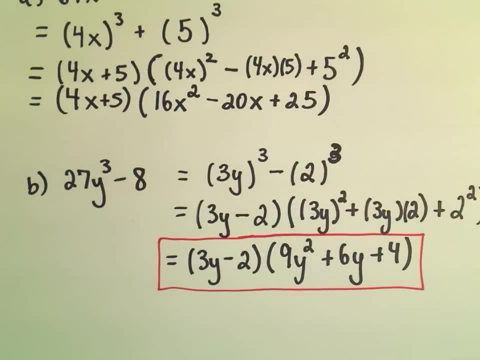 maybe in a pre-calculus class. There's certainly formulas that people forget. So even if you forget it, at least know that there is a formula out there, And that way, if you're doing a homework problem or something, at least you'll know. 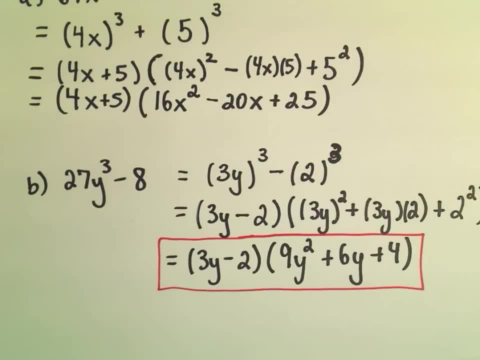 oh hey, you know I should dig out my algebra book and look it up. So again you know, just a little practice, but again nothing too crazy. Just a few more formulas that unfortunately you got to know.